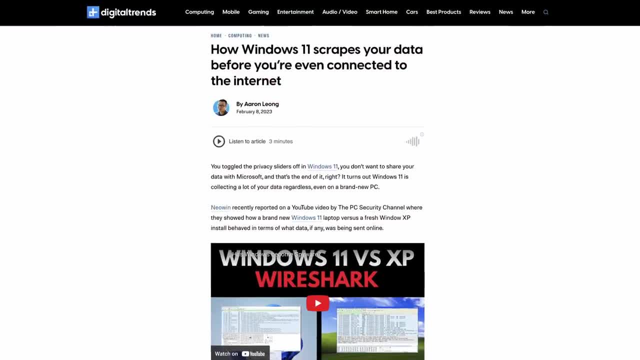 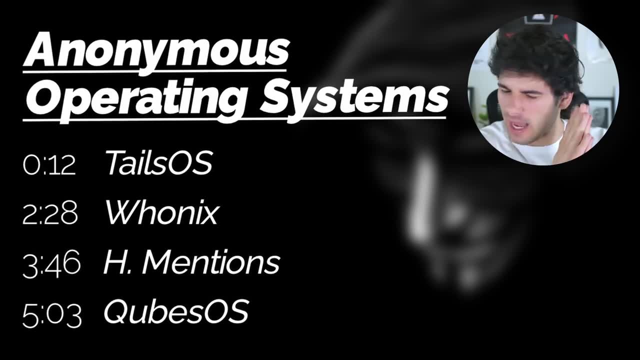 Most operating systems aren't anonymous. Hell, most don't do the bare minimum of not tracking you. Today, I'm going to share three of the world's most anonymous operating systems for people needing the highest degrees of protection. TailsOS is a Linux distribution which runs as a 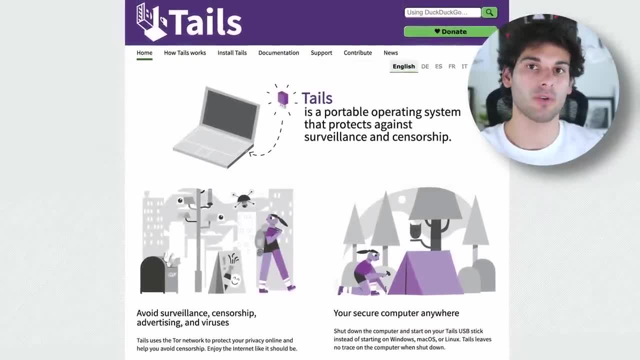 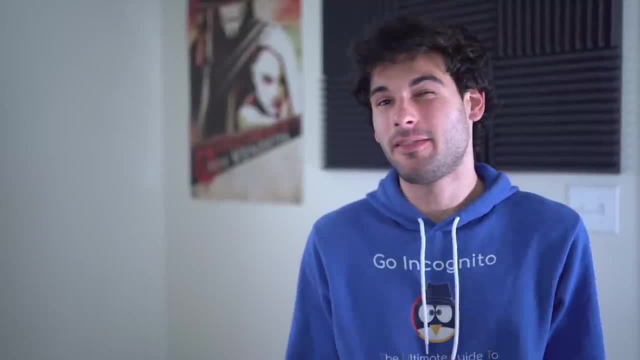 live operating system, meaning it's never installed on your computer, but rather on removable storage like a flash drive which you boot into from any system. Now I really like live operating systems, not even necessarily from a privacy and security perspective, but just. 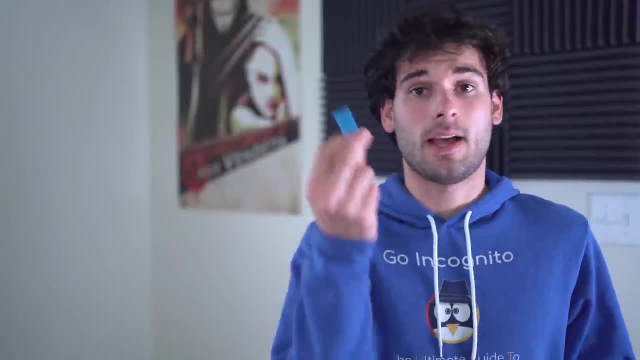 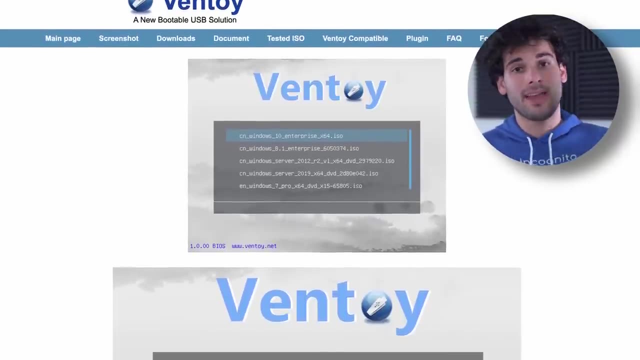 from a usability perspective. For example, I can carry a flash drive that has VentoyOS and this can hold like five different live OSs or however many I want, and then the other one can run TailsOS. And so anywhere I'm in public, on any computer, I can boot into an operating system. 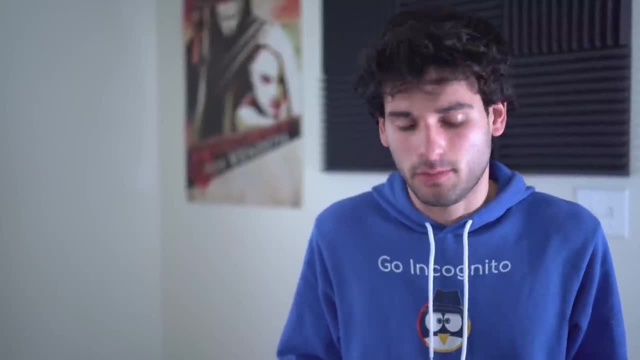 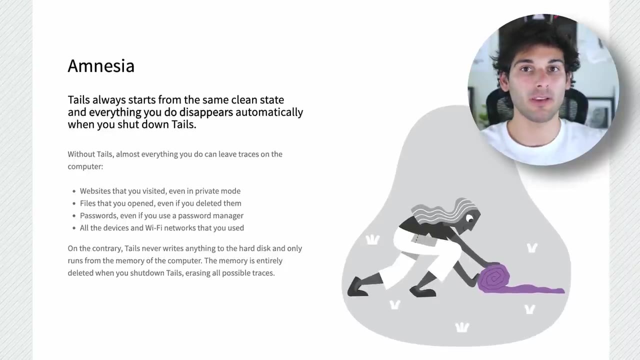 of my choice, which is really cool just from a pure usability perspective. So I really like live operating systems. aside from their designed use case of testing Linux, By default TailsOS is non-persistent, so any installations, files, settings and other things that you want to. 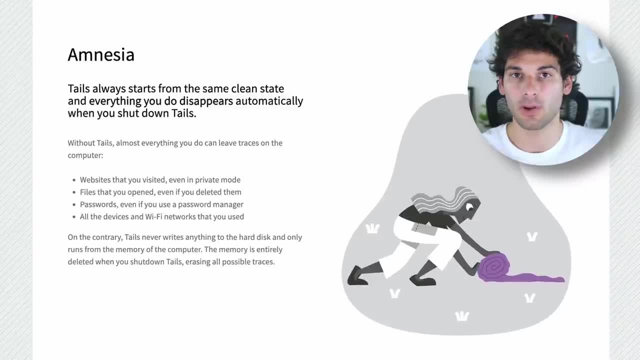 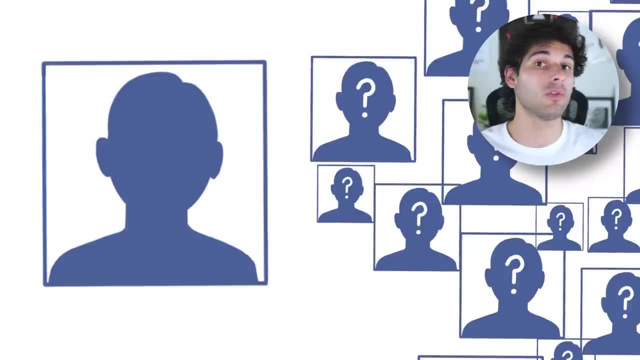 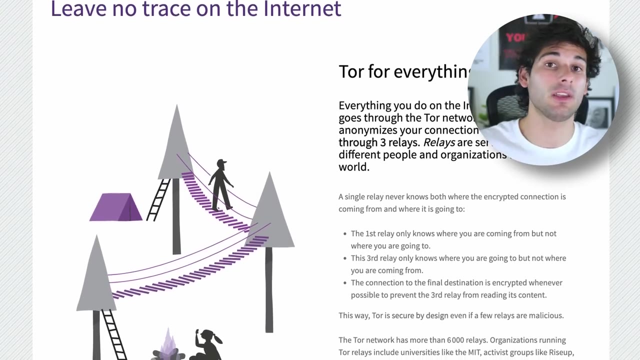 change are automatically wiped when you shut down, where the flash drive returns to factory defaults. What really separates Tails is its integration with countless anonymity tools and configurations to make you blend in with everyone else using it. Everything from software updates to your web traffic is routed through the Tor network. Your device's unique MAC address is booted by. 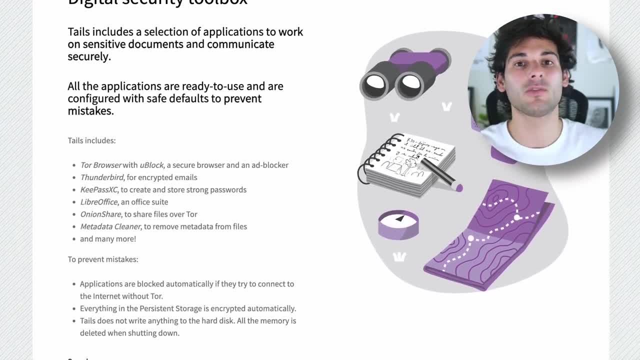 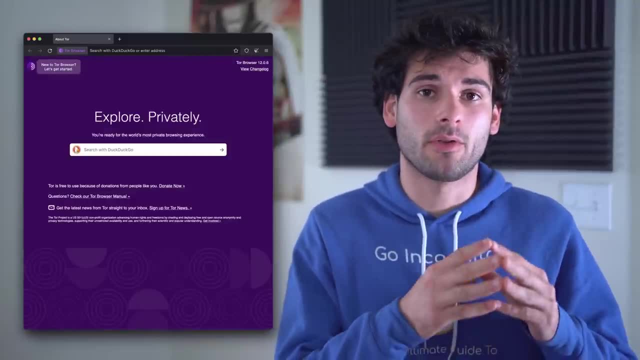 default, it includes a tool that strips metadata from any file, as well as countless other tools you can dig into. Now, the anonymity of TailsOS is pretty unique, so traditionally when you use the Tor browser, you are anonymous within that session and you're pretty much getting 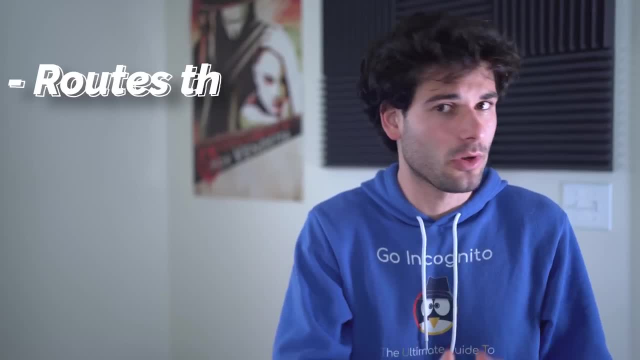 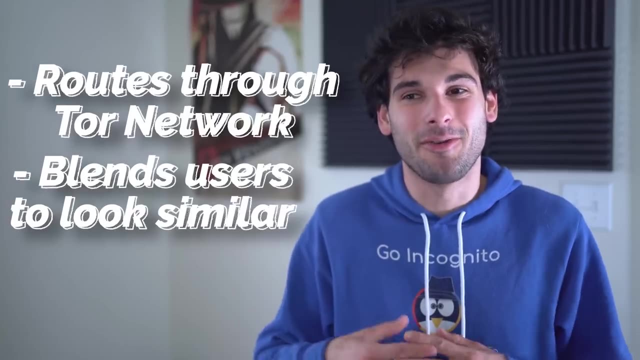 two layers of protection. Everything you're doing is routed through the Tor network, which a lot of people seem to understand, but the other very important piece is that every Tor browser user is meant to look the same, So it looks like it's the same person who's accessing the Tor network. 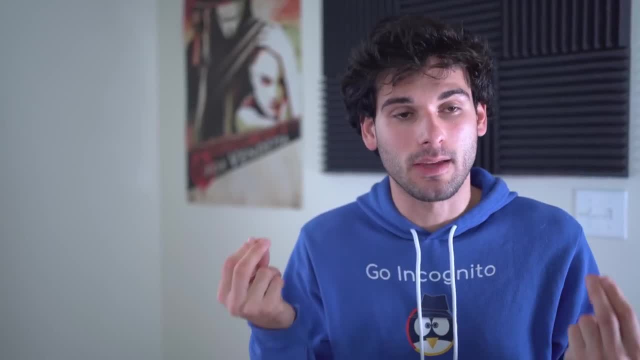 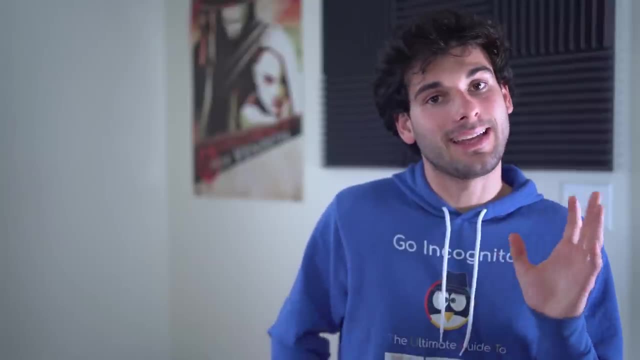 The Tor browser is then effectively a tool that accomplishes two things: It's designed to make people look the same, and then it routes you through the Tor anonymity network. TailsOS is special because it extends that protection around the Tor network, And then it also allows you to. 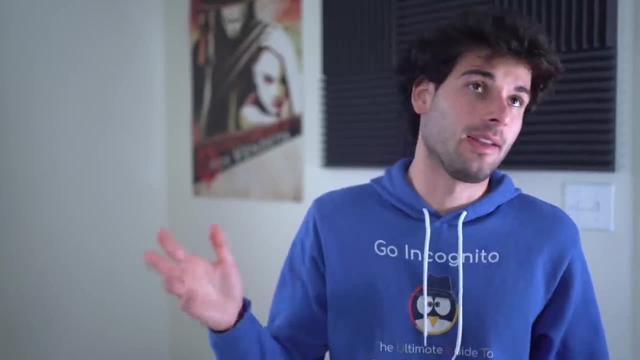 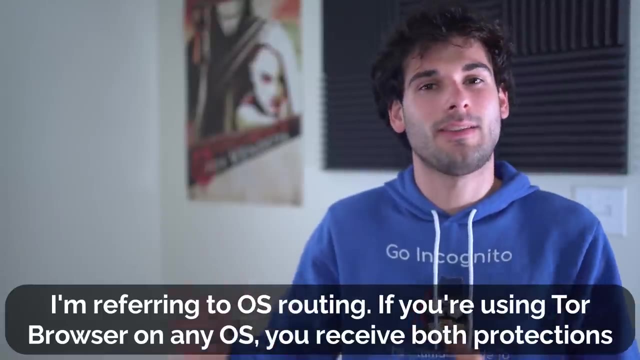 onto an operating system basis. Just to summarize that if you run like a normal operating system, like Windows, Fedora or whatever you want, through Tor, you kind of get half of Tor's protection in a way. you're missing out on the blending in. 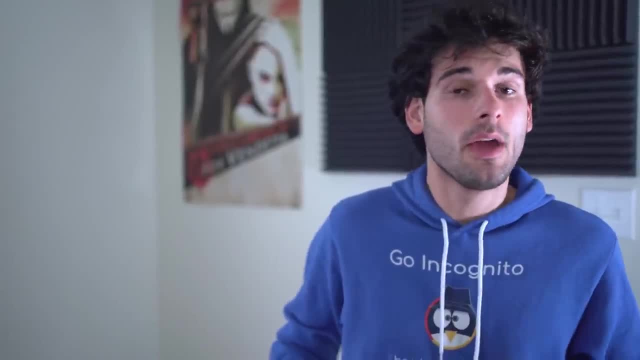 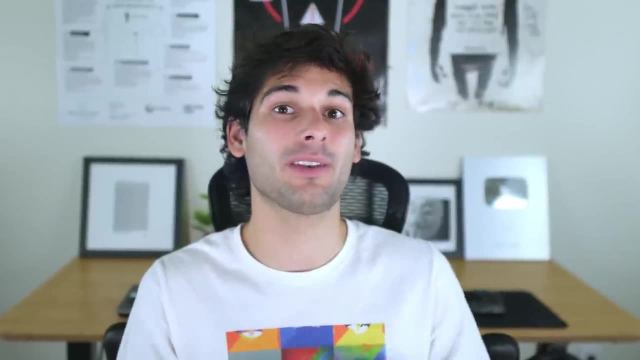 with everyone else, aspect of Tor which might be fine for certain threat models. but Tails OS does kind of both things, where it blends you in and it routes you through Tor. All these attributes make Tails OS one of the best choices for users. 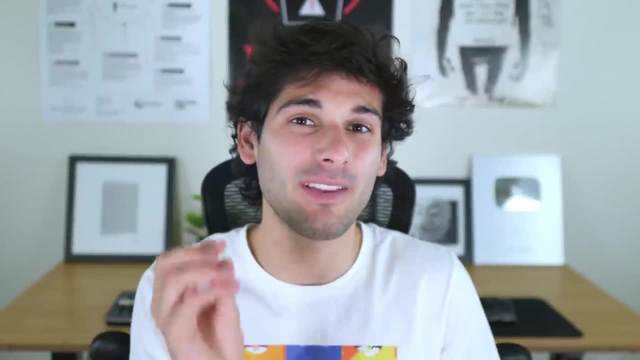 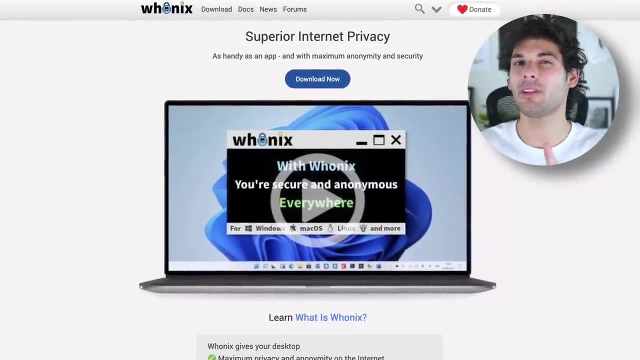 needing the highest degree of anonymity, all in a package that fits in your pocket. Next is Hoonix, an OS with the goal of anonymity and security, but originally with an emphasis on being a virtual machine. A virtual machine is an operating system. 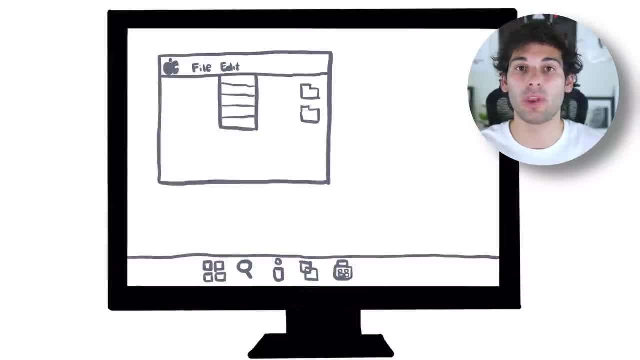 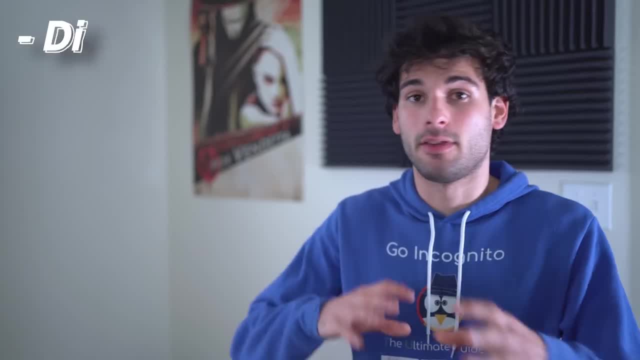 that runs virtually on top of your normal operating system. in real time Virtual machines are awesome and they're actually again kind of like live operating systems: a staple. just for my usability, I can have different virtual machines for different workflows and different purposes. 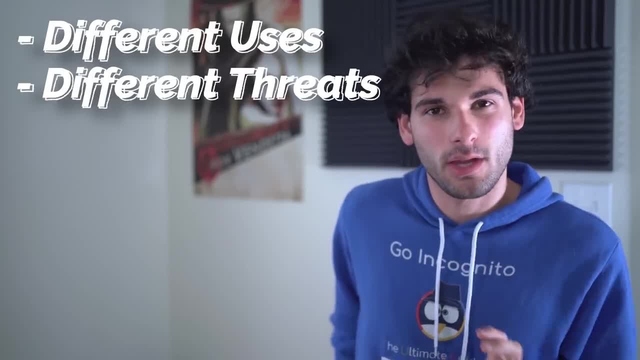 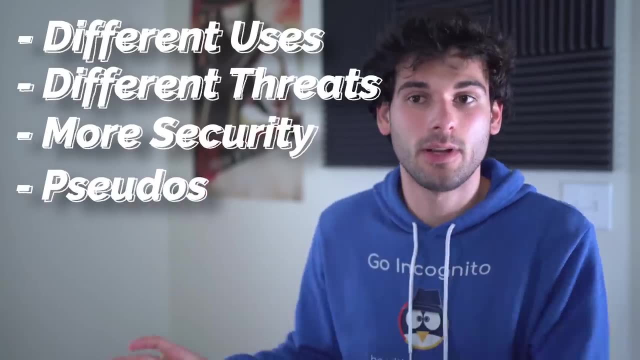 for different threat models. If there's something that needs a little bit more security, I can make sure I have my downloads and things that are a little bit riskier done inside a virtual machine. I can have a virtual machine designed for a pseudonym. 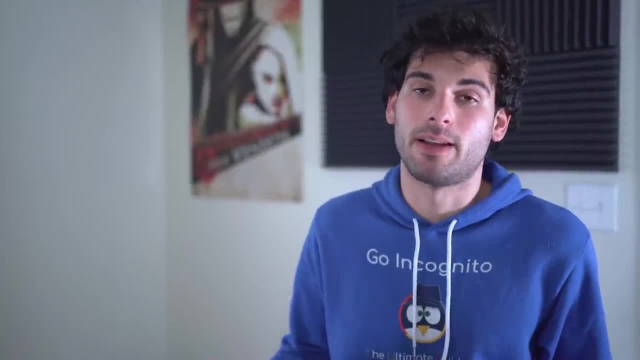 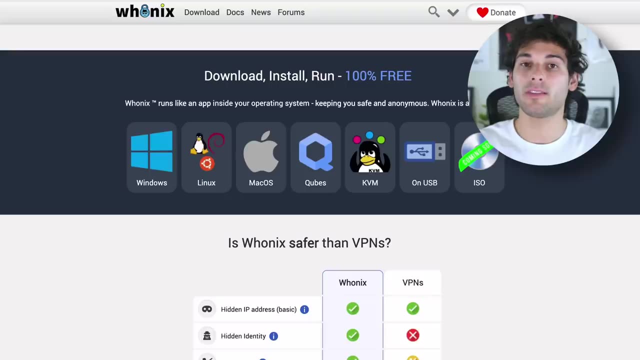 I can have a virtual machine for really anything I want, So it's cool to have Hoonix run as one of these, because then it's just one more virtual machine in an already extensive sandbox that you have available to you. This is nice, as it reserves anonymity. 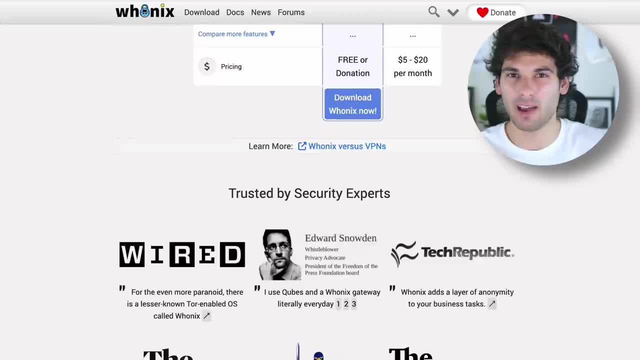 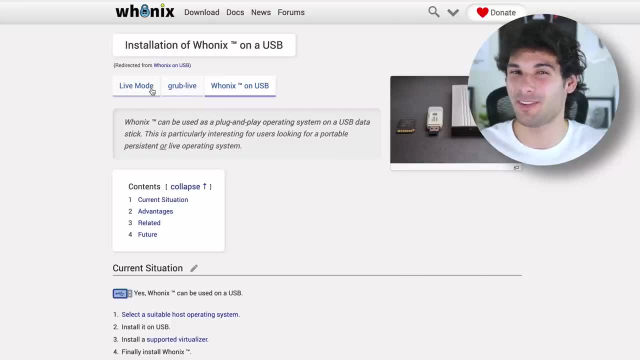 only for when you need it on your normal system, not all the time. While this is their most popular offering, Hoonix recently introduced a live version similar to Tails, so we have a little competition here. If you're wondering if Hoonix compares to Tails, 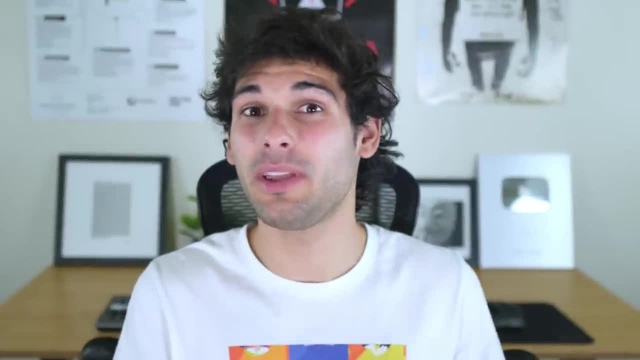 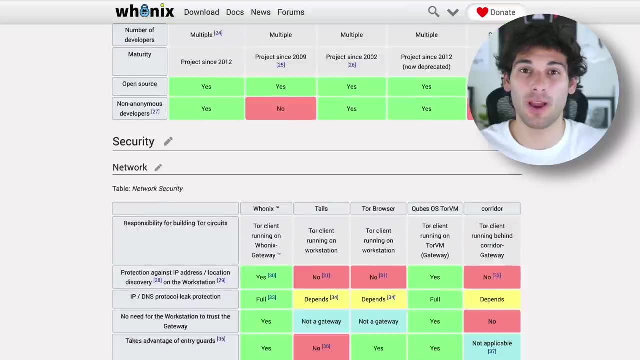 especially the live versions. ultimately it's complicated and really depends on your needs, But despite this comparison coming from Hoonix, it's pretty darn objective and honest about each OS, So we encourage using this chart to compare Hoonix to Tails. after the video is done: 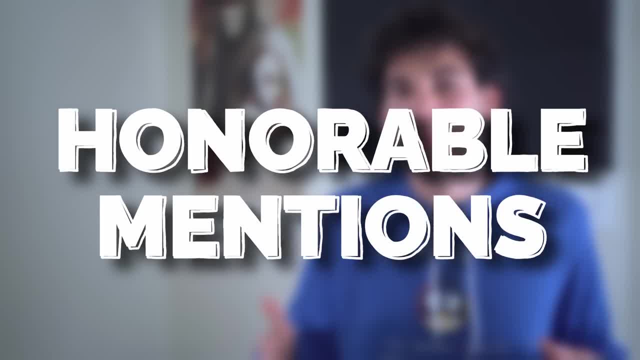 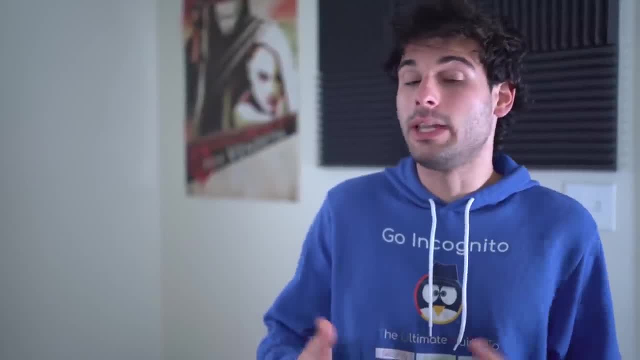 to see which is better for you. Now a few honorable mentions, but mainly a quick note before I cover the last and final operating system. I wanna mention that most people who watch this likely don't need to be using these powerful operating systems 20 years. 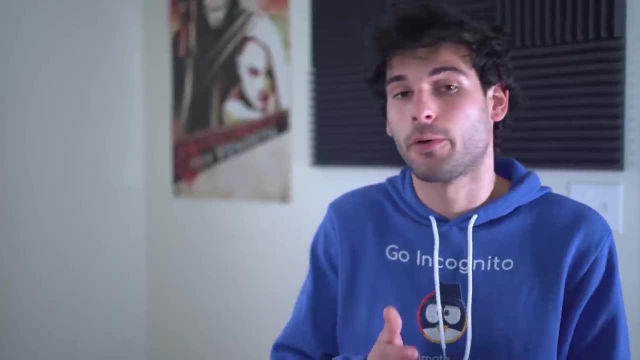 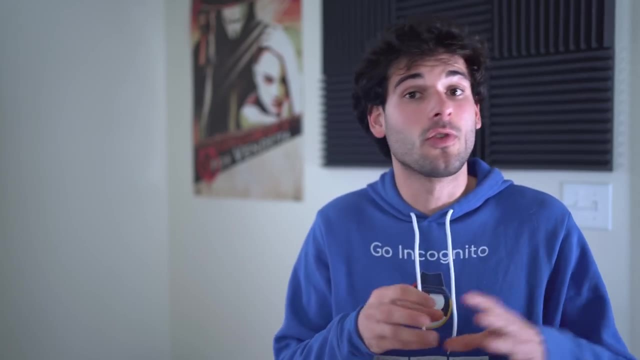 24, seven, And most of you can probably just get away with using them just for specific use cases that need their safety, And I don't really believe in black and white privacy. I think that there are specific situations where you need more privacy and more security. 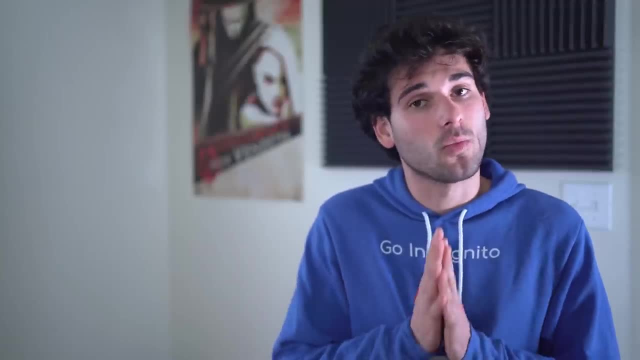 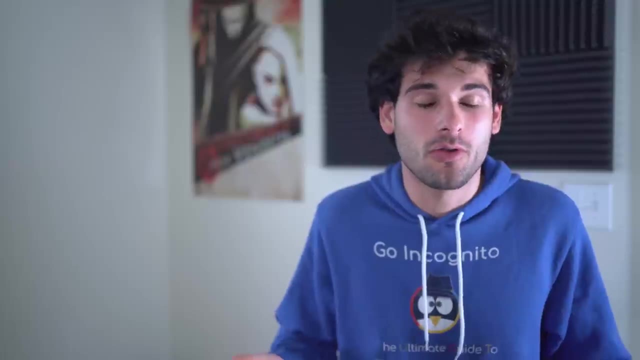 and some situations where you don't, And it's fine to make that compromise when you can. If you can't make that compromise, then yeah, don't make the compromise. But again, this is why it's a pretty individual journey And I try to stay away from the black and white mentality. 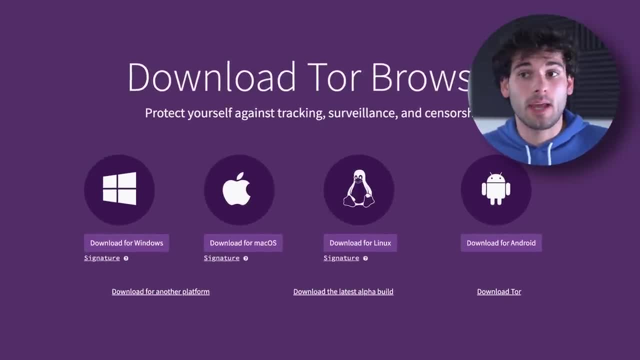 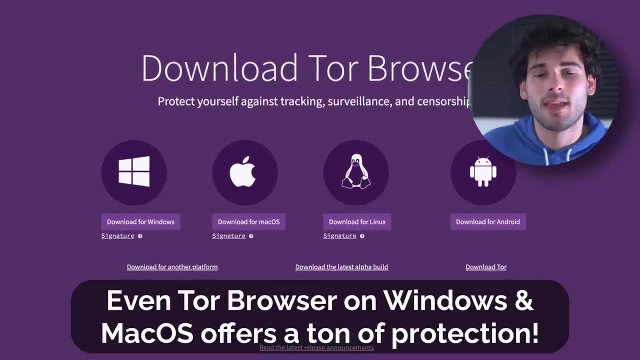 I often see in the privacy world. As an extension of that, I wanna mention call out: just using the Tor browser on your standard operating system already offers a huge layer of protection within that operating system, especially if you're keeping everything you're doing inside the browser. 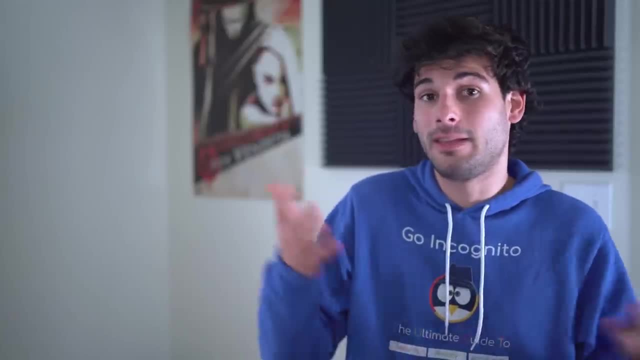 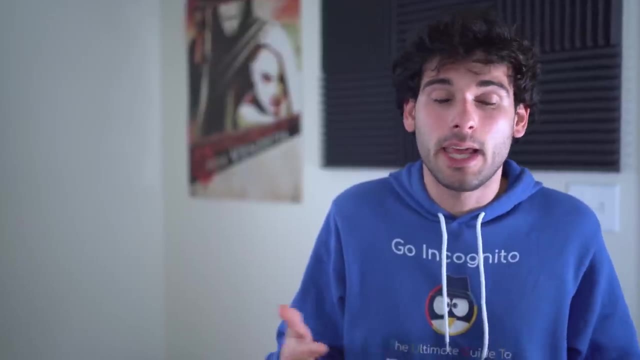 And so your honorable mentions do ultimately come down to things like Fedora, OpenSUSE, Arch and most other Linux distributions that allow you to use this incredible Tor browser in a fairly safe and privacy respecting environment. that should fit most people's threat models more than enough. 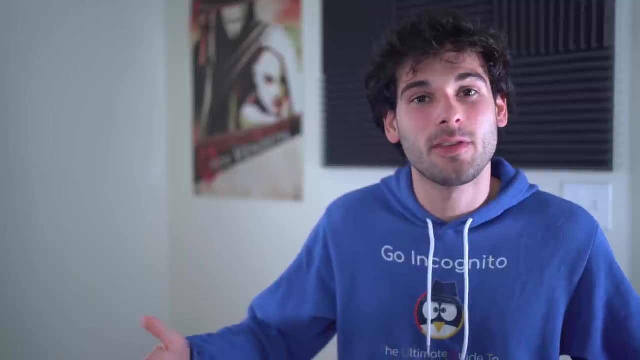 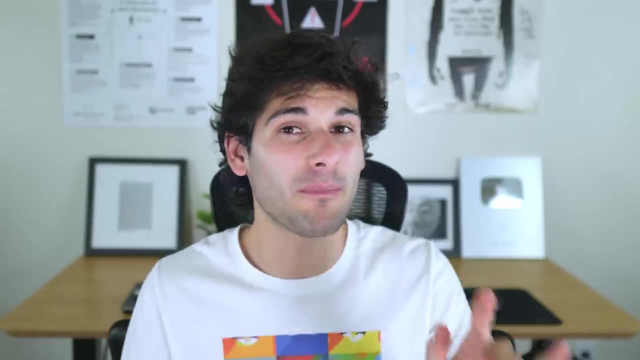 Again, if you need more, then that's why I'm covering extensive options, but sometimes don't forget the basics, because for a lot of you that might actually be more than enough. Now, the final operating system is unique for a big reason. 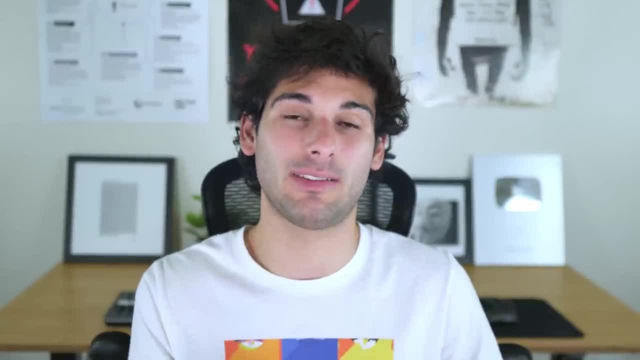 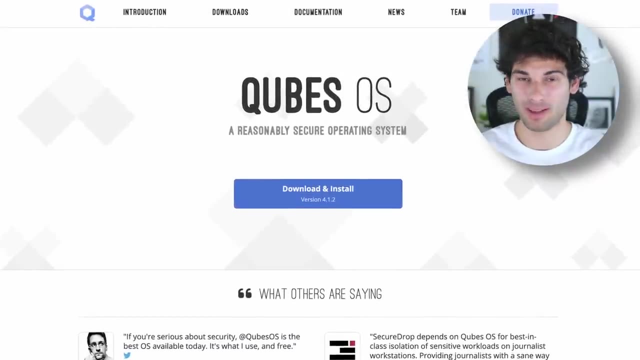 It's designed to be used as a daily operating system. Cubes is based on Zen and Fedora with the goal of security by virtualizing pretty much everything as its own compartment Out of the box. Cubes doesn't inherently offer greater degrees of anonymity. 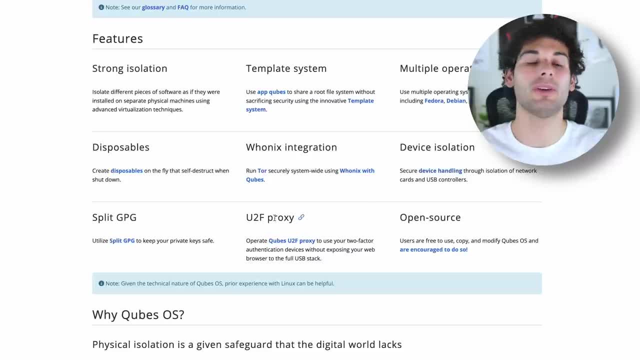 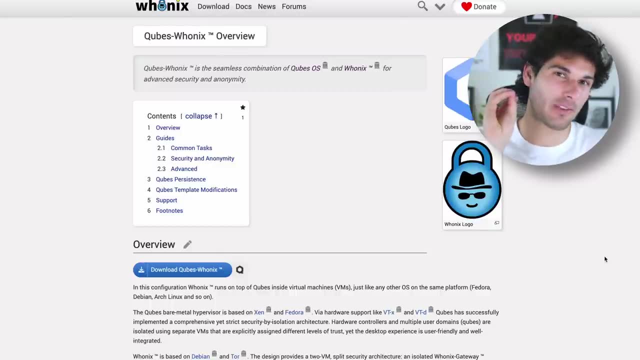 compared to your typical OS at least. but that quickly changes when you begin looking at the VM options within Cubes, including an option for Tor VM and, yes, a Hoonix one as well. So if you liked Hoonix but want Hoonix to run, 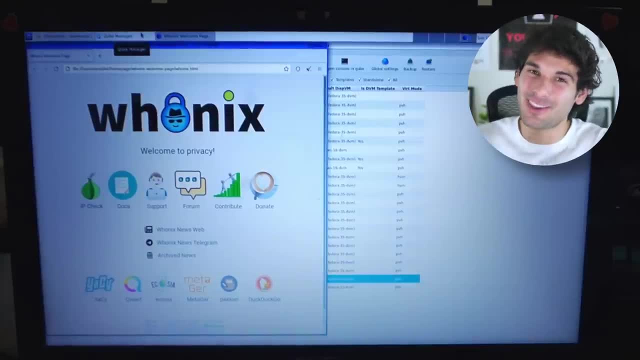 on top of a much more secure and trusted operating system. Cubes is the way to go, as it combines all the positives of Hoonix, but on top of a more secure OS. The cool thing is, while Cubes is a bit clunky to use, 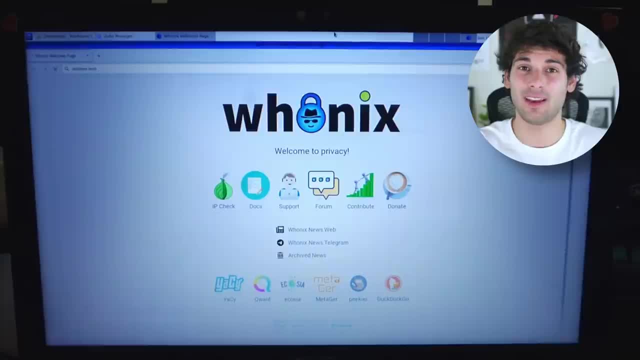 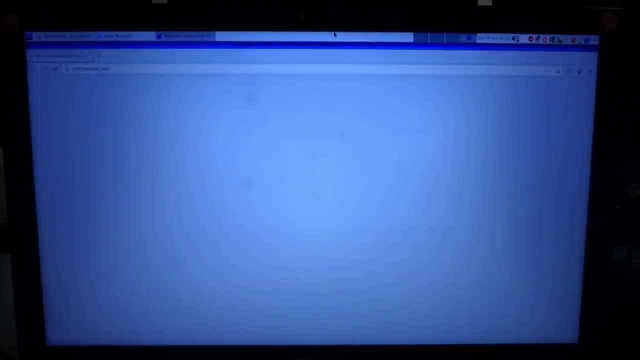 it's not super unrealistic for technical folks to use it. Oh, folks, Folks, technical folks. It's not super unrealistic for technical folks to use it as a main OS day to day. It allows you to easily keep things like Hoonix. 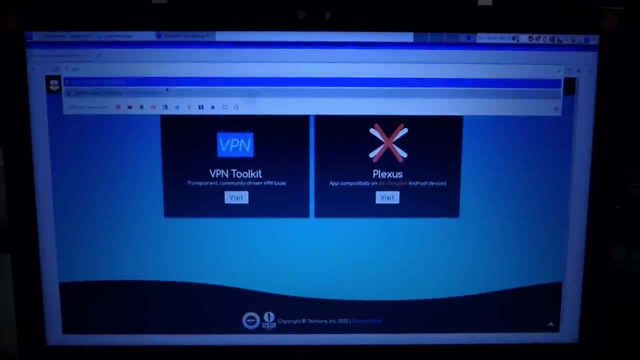 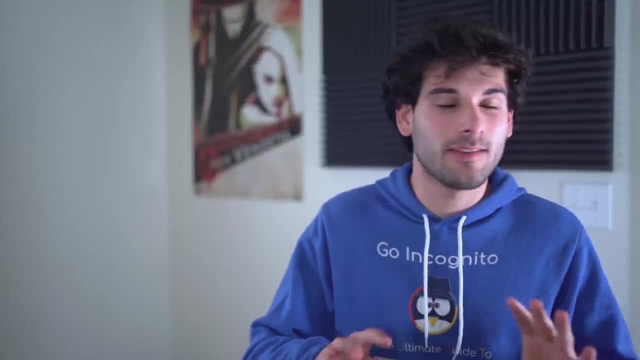 safely reserved for when you actually need the anonymity and it gives you the option to use normal things day to day that don't need the anonymity. And a quick note on Cubes, aside from it being seen as a privacy and security tool similar to virtual machines. 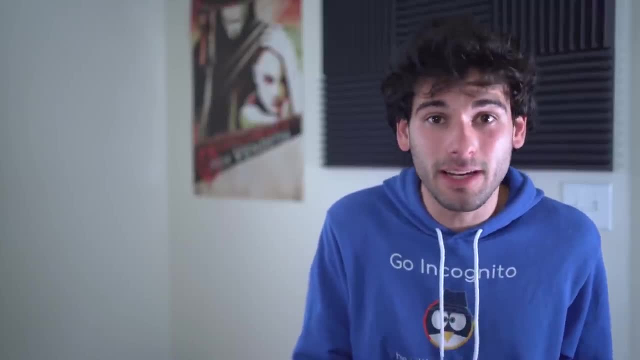 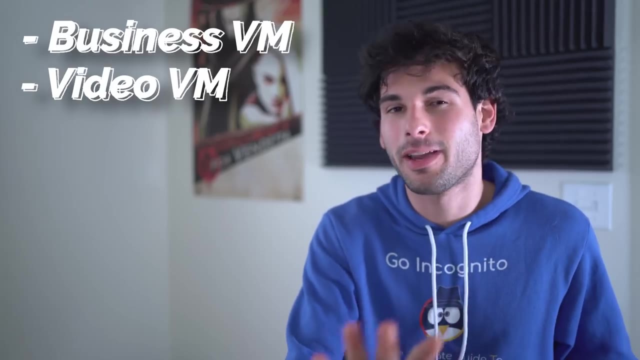 this compartmentalization is actually a really cool use case and usability tool. So you can have like whole businesses run on just one VM And Cubes, or you can have video production. I wouldn't recommend producing videos in Cubes, I think that's insane. 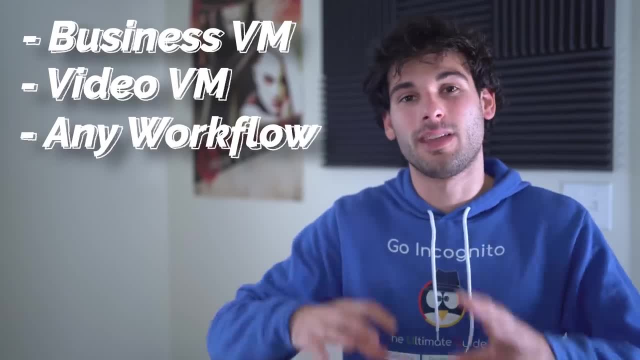 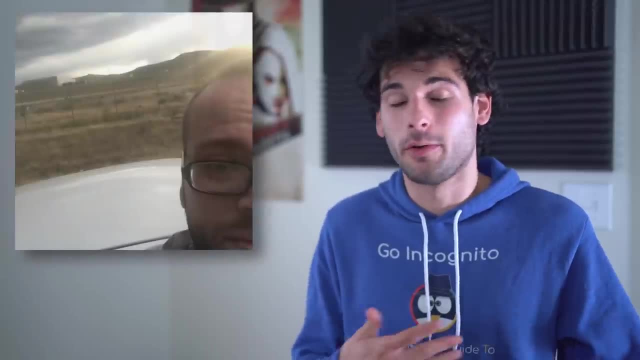 But like as an example you can have, like straight up workflows in your life, only done in a single part of Cubes- And Cubes is, from a usability perspective, allows you to do that very cleanly. Nate, who I co-host on surveillance support. 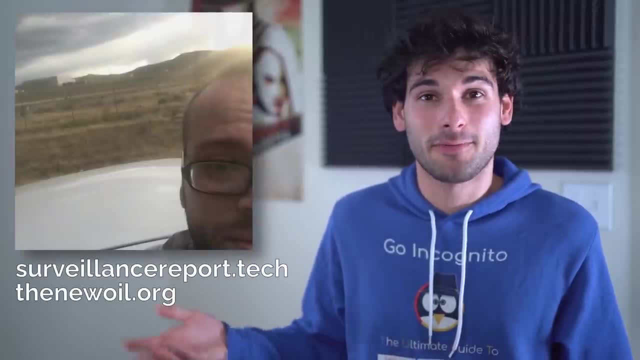 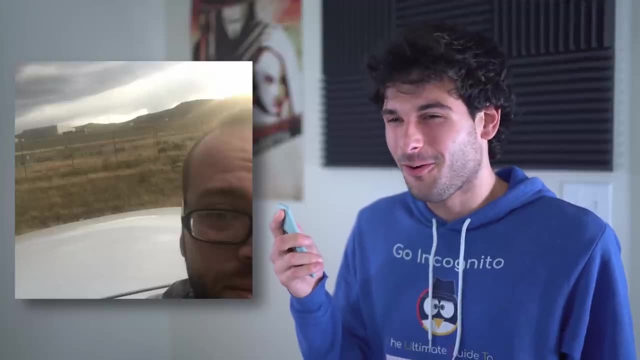 is a big shill of Cubes and uses it for a ton of things. And he says: for usability, All right, what's the question? I'm recording something. What do you like about Cubes? Why do you use it? Why do you use it? 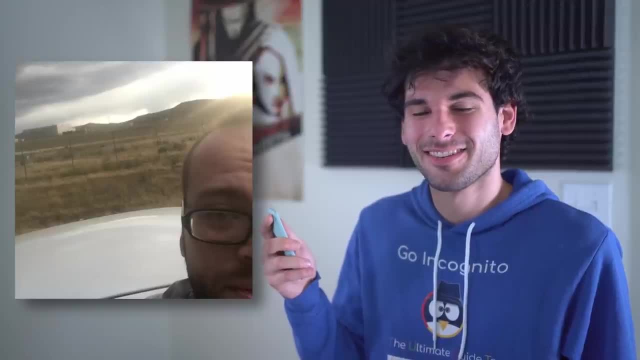 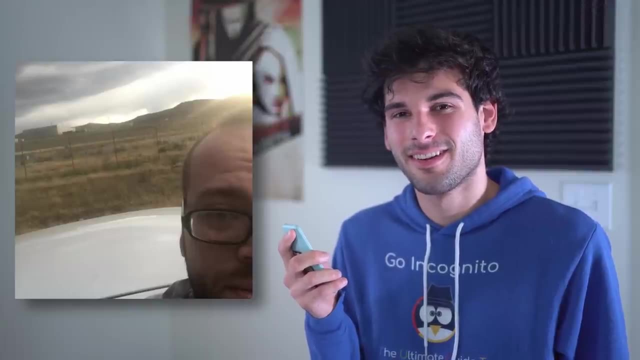 Okay, I enjoy the isolation. I enjoy that it makes it really easy to keep track of multiple accounts, like multiple signal accounts, multiple matrix accounts. I don't have to use different matrix clients. I can use the same client over and over. 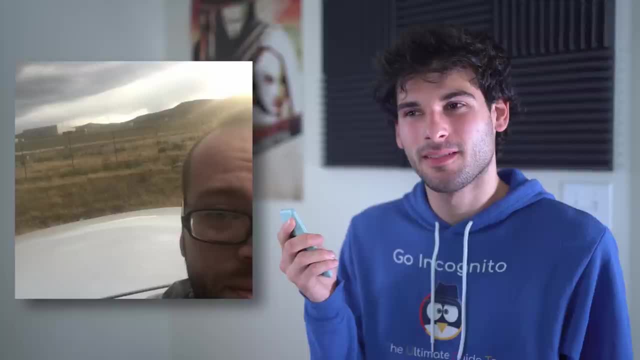 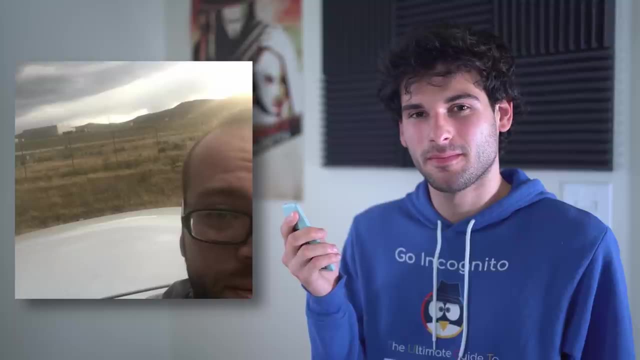 And I like that. it makes it basically impossible to send the wrong thing to the wrong person. You can't really copy and paste. You know a link that wasn't meant for a different identity or something like that. I like the fact that I can compartmentalize. 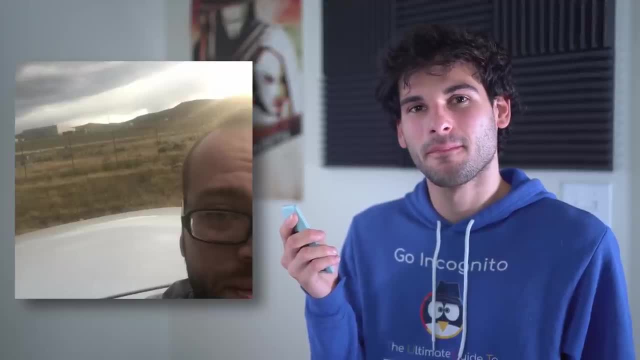 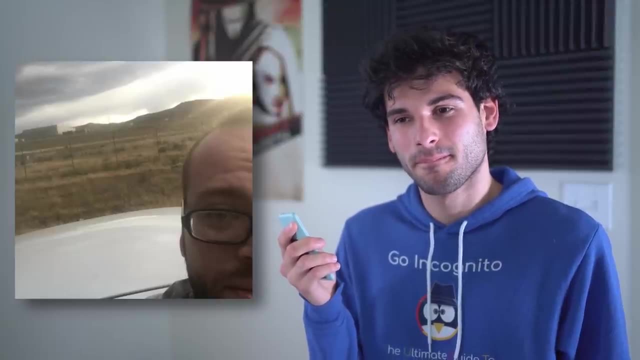 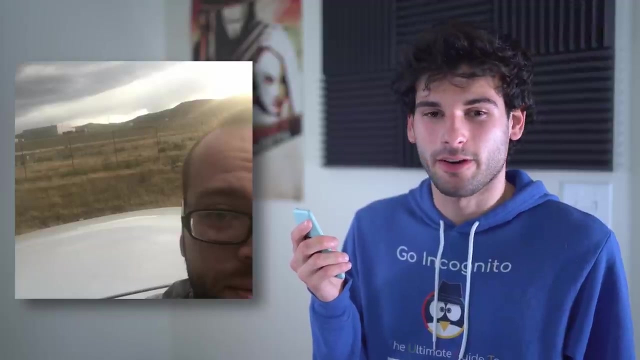 and reduce the risk of any sort of crossover or possible infection. I can spin up temporary VMs with one click to open links and attachments. I think those are kind of my big points. So it sounds a lot like a usability thing, almost Like, yes, it extends into security and privacy. 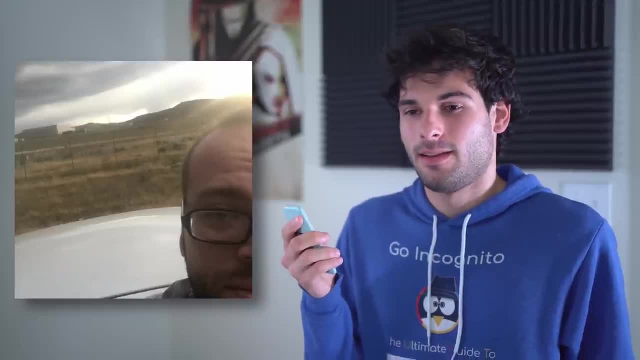 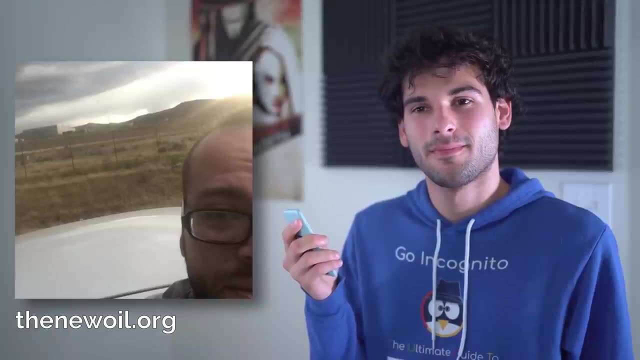 but you almost like the usability of it in a way. Yeah, I mean, for me personally, cubes is actually like super overkill for my threat model. I probably don't need it, but for me it really gives me a lot of peace of mind. 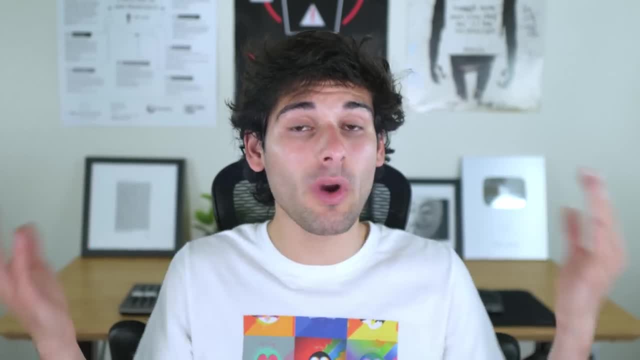 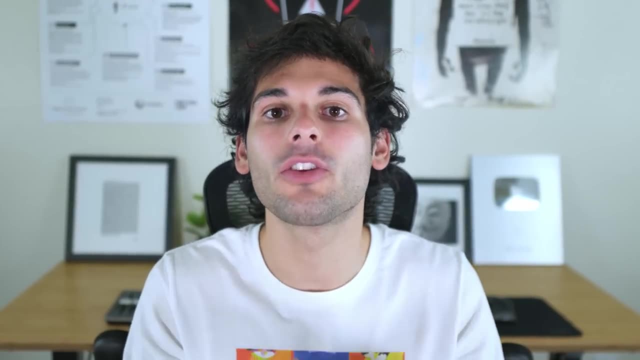 and really improves my workflow. All of these are incredibly powerful tools that enable people like you to be safer online, So take advantage of what they offer. They're incredible tools. Download them and play around, And I promise you're gonna learn a lot in the process. 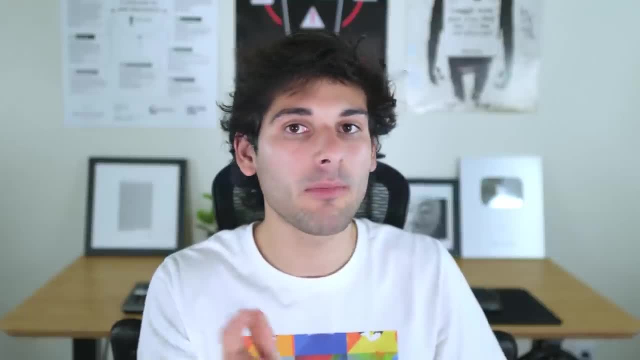 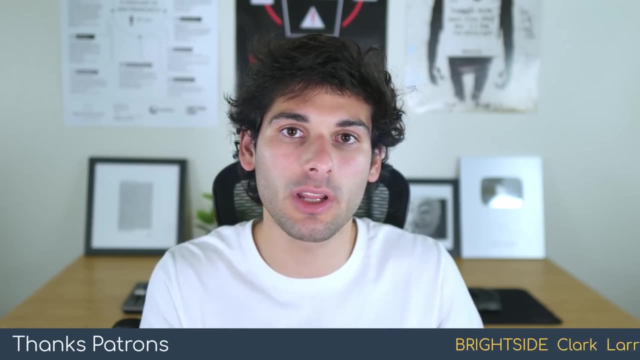 and you're gonna enjoy them a lot. With that said, like most tools, you have to use them properly. If you want to learn more about how to use these tools and how they fit into your privacy and security journey, check out our Become Anonymous guide right here.